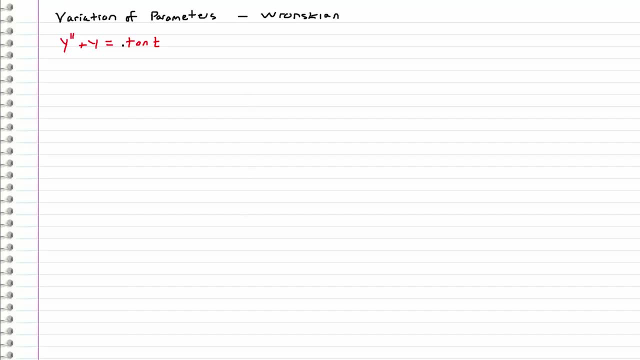 Hey guys, welcome back to our last video on variation of parameters, where I'm going to show you a little quick trick to finish the problem faster. So in the last videos I've showed you this really tedious process of determining u1 and u2, but instead now we're 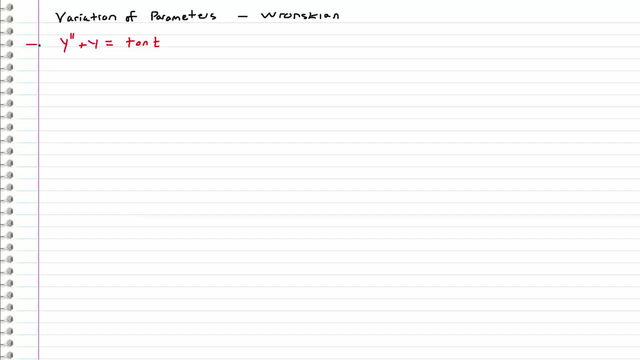 going to look at how to do that using the Wronskian. So let's revisit this example right here. y double prime plus y is equal to tangent t and we determine that the homogeneous solution of this is equal to c1 times cosine t plus c2 times sine t, And normally for variation. 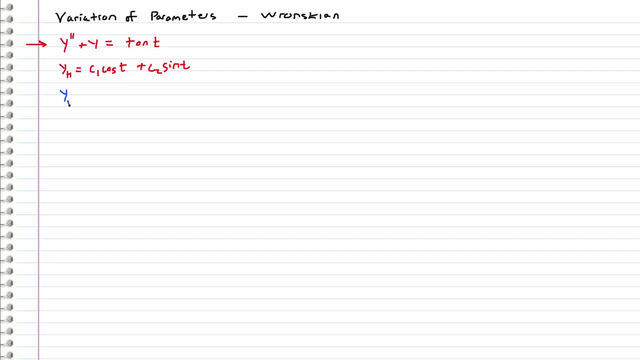 parameters. what we do is we drop the c's and add the u's, so we assume the particular solution of the form u1 times cosine t plus u2 times sine t, where u1 and u2 are functions of t. So, without going through that tedious process to determine u1 and u2, we are going. 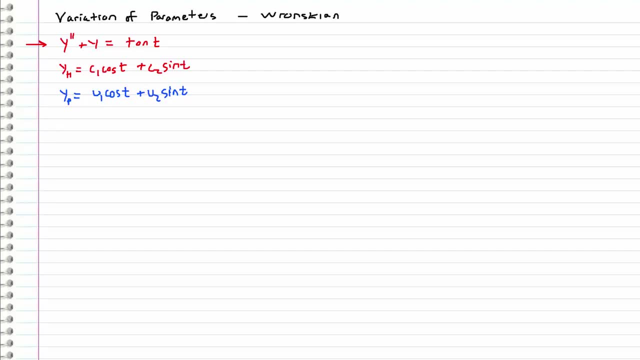 to compute them directly using the Wronskian. So here are the functions of t. Here are the formulas that we will be using. We have: u1 is equal to the negative integral of y2 times f of t over the Wronskian, and u2 is equal to the integral of y1 times f. 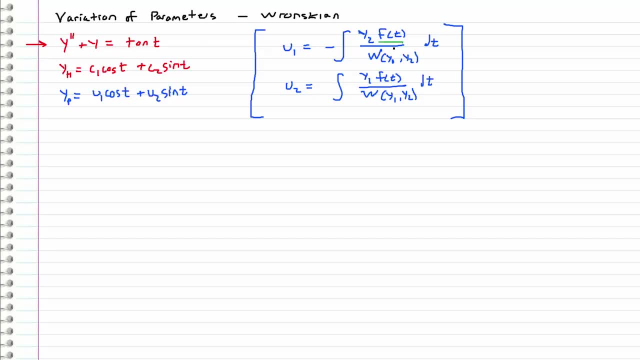 of t over the Wronskian. So what I mean by f of t is just the non-homogeneous part of the difference equation. So this guy is f of t And what I mean by y1 and y2, these are just the first and second homogeneous solutions. So this would be y1, and this would 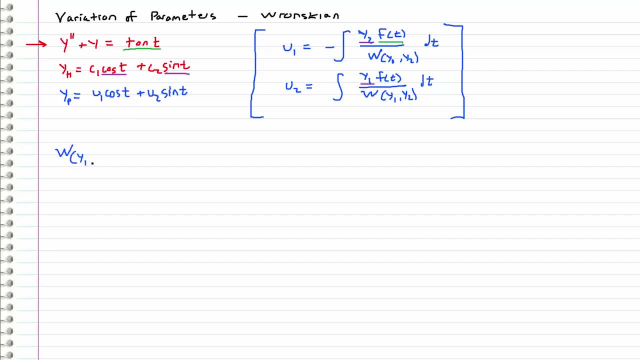 be y2.. And then, of course, the Wronskian of y1 and y2 is equal to the determinant of y1 and y1 prime, and then y2, y2 prime. So let's go ahead and use these formulas to determine. 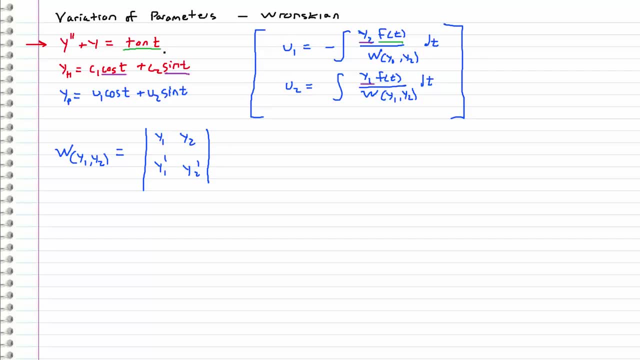 u1 and u2 directly and solve this non-homogeneous difference equation. So let's start off by evaluating the Wronskian. So let's go ahead and replace y1 and y2 in this formula, So y1 is cosine t, y2 is sine t and they're. 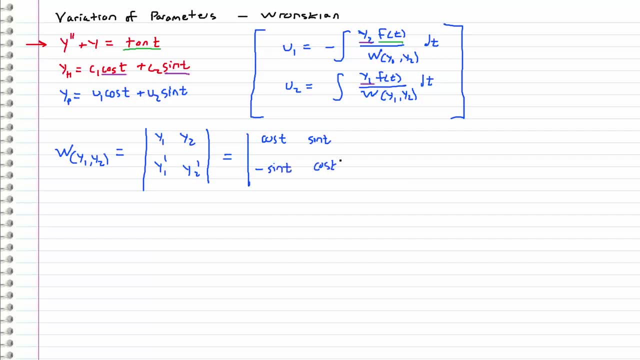 derivatives are negative sine t and cosine t respectively. So when we take the determinant we get cosine squared t and then plus a sine squared t, which we know is just equal to 1, from that common trig identity, And so we have everything we know to evaluate these. 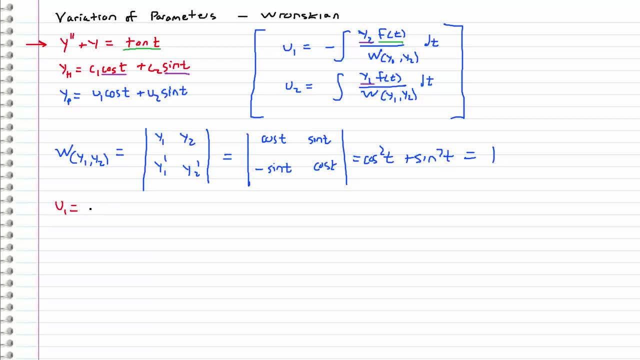 integrals now. So let's start with u1.. So u1 is equal to the negative integral of y2, which is sine t times f of t, which is tangent t all divided by the Wronskian of y2, and. 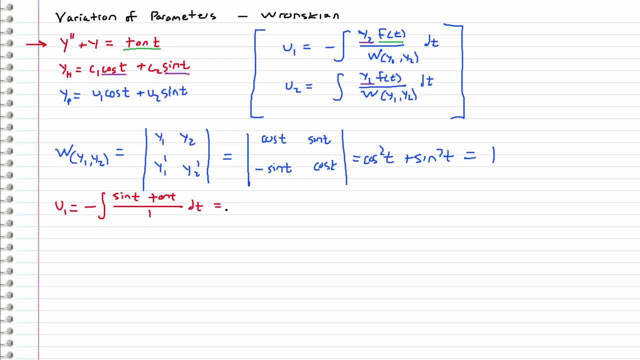 which is just 1 dt. So this is the same integral that we encountered last time, where we used a trig integral identity, And we're going to use the same thing here. So this comes out to be the negative natural log of secant t plus tangent t and then plus sine t, And 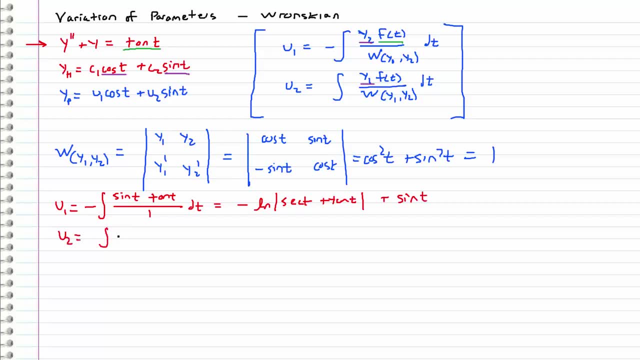 then our u2,, which is equal to the integral of y1,, which is cosine t times f of t, which is tangent t all over 1 dt. This is just equal to the integral. The cosine cancels with the cosine and the tangent, leaving 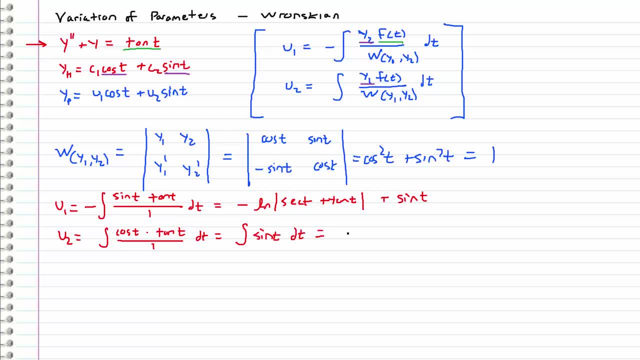 just a sine of t, which we know to be negative cosine t. So we have already computed u1 and u2, and we've saved a bunch of time And we are already ready to assemble our final solution, which is the homogeneous solution plus the particular solution, So plus u1, which is 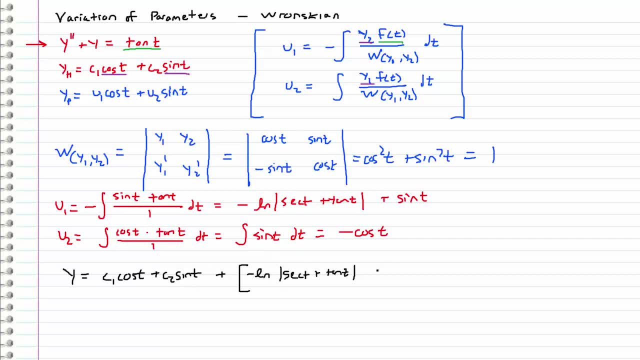 this mess all times cosine t and then plus u2 times sine t, which is minus cosine t times sine t. And this guy cancels out with this guy, since it's being multiplied by a cosine And that leaves us with just: y is equal to c1 times cosine t plus c2 times sine t minus. 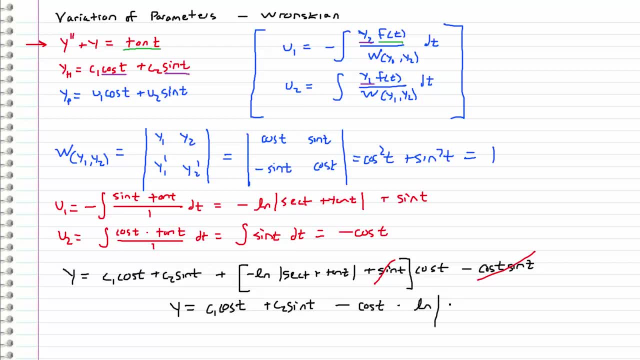 cosine t times the natural log of secant t plus tangent t. So this is our answer, And look at how fast we did that. It almost makes you frustrated that we went through all that trouble in the last video. But as I understand it, some professors 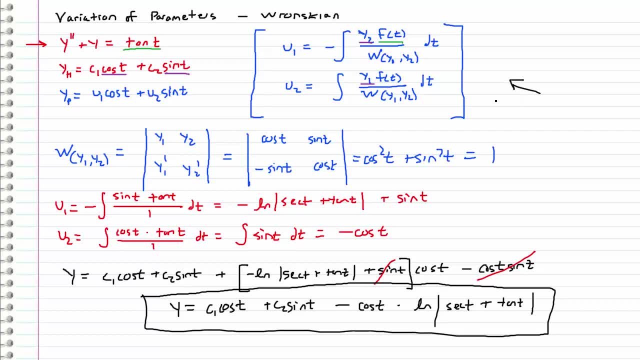 prefer you to use this method and some professors prefer you not to use this method. Personally, whenever I took differential equations, my professor said, no, you're not allowed to use this method, So I never used it, but maybe you can. So anyway, thanks for watching and I will see you guys later.